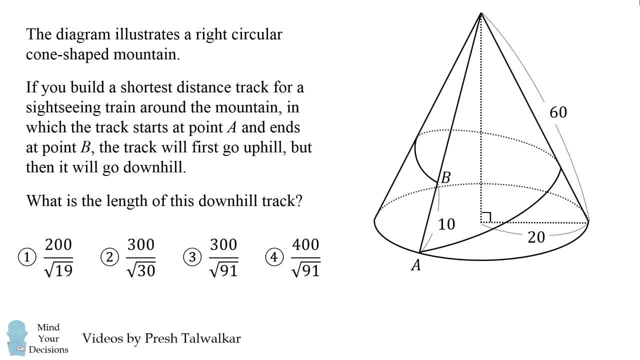 And 400 divided by the square root of 91.. So I will say this problem was very challenging for me. But can you figure it out? Give this problem a try and, when you're ready, keep watching the video for a solution. 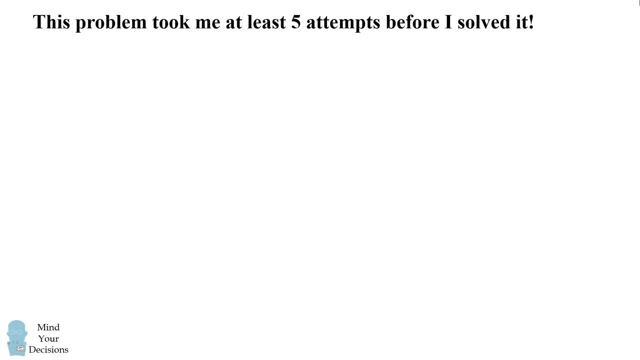 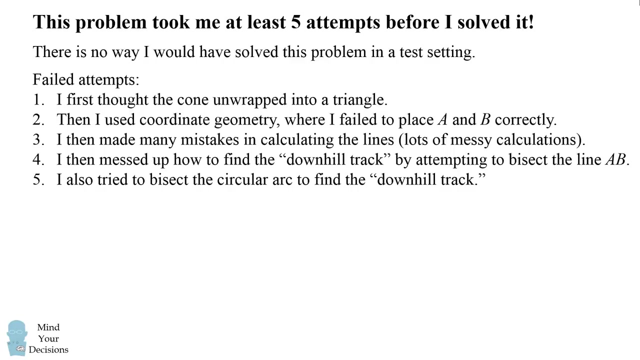 So this problem took me at least five attempts before I solved it. There is no way I would have solved this problem in a test setting. And here are some of the failed attempts. I first thought the cone unwrapped into a triangle. Next I used coordinate geometry, but I failed to put the points A and B in the correct positions. 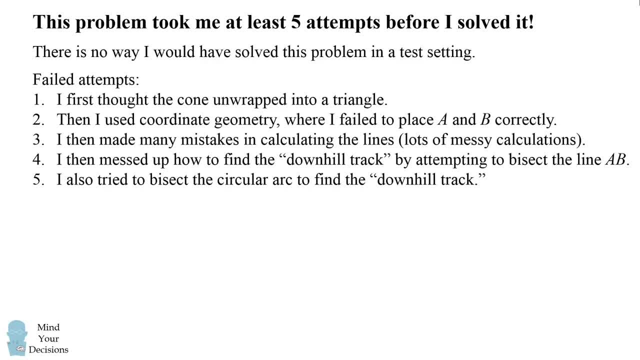 The third mistake is that I then made many mistakes in trying to calculate the equations of the lines. This led to many messy calculations. The fourth mistake is that I messed up how to find the length of the downhill track, because I tried to do it by bisecting the line AB. 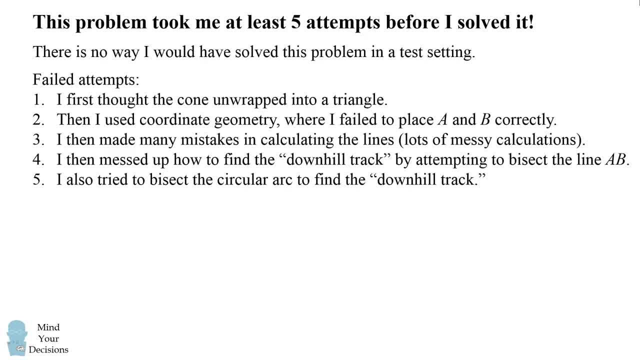 This is not correct. I then tried to solve it by bisecting the circular arc to find the downhill track. So I was stuck and then I said maybe I should try and find the answer on line. But then suddenly it hit me. Eventually I figured it out. 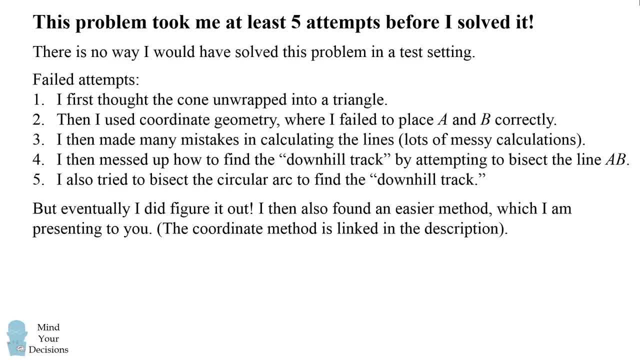 I found an easier method to solve the problem, which I am presenting to you. The coordinate method is linked in the description, So why am I sharing this story with you? The lesson is that don't give up if you can't solve a problem, And also don't peek at the video solution too early, Challenging problems often. 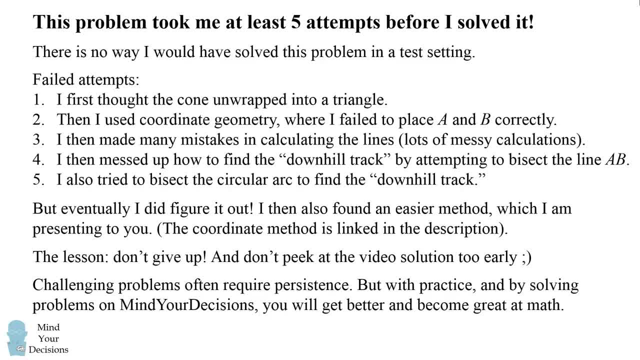 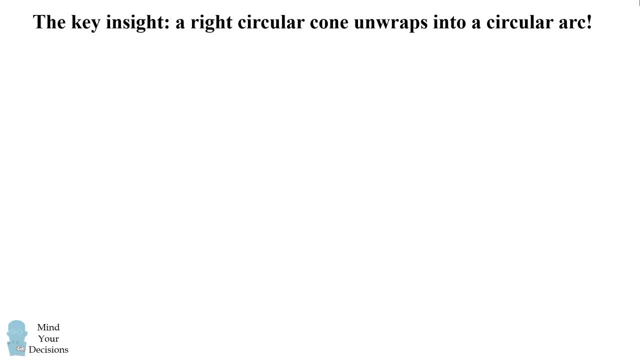 require persistence, but with practice and by solving problems on mind your decisions, you will get better and you will become great at math. So how do we solve this problem? The key insight is that a right circular cone unwraps into a circular arc. 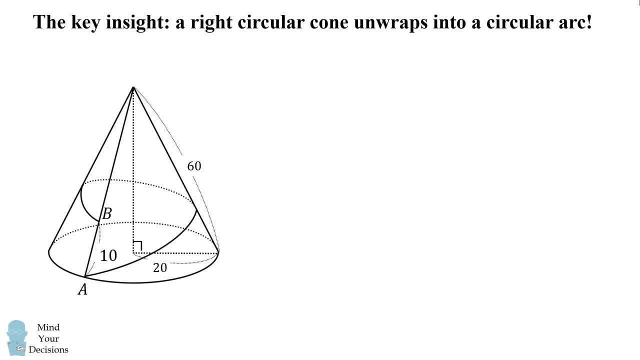 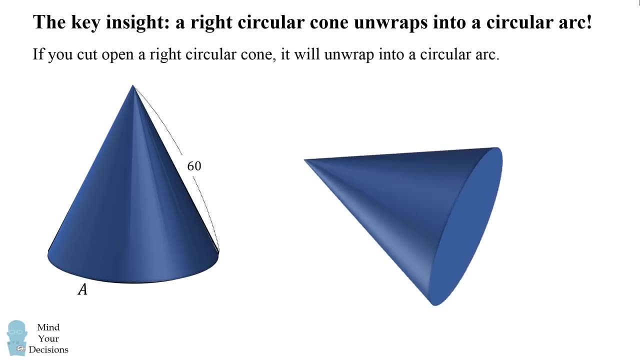 So here we have the cone-shaped mountain and let's just imagine a general cone. If you cut open a right circular cone, it will unwrap into a circular arc. So here's a visualization of what I'm talking about. So we have this cone and it's a three-dimensional object. 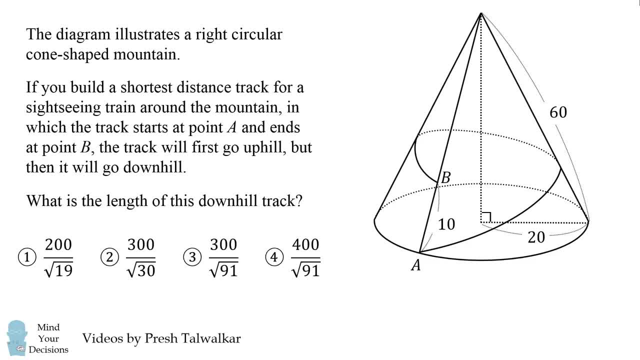 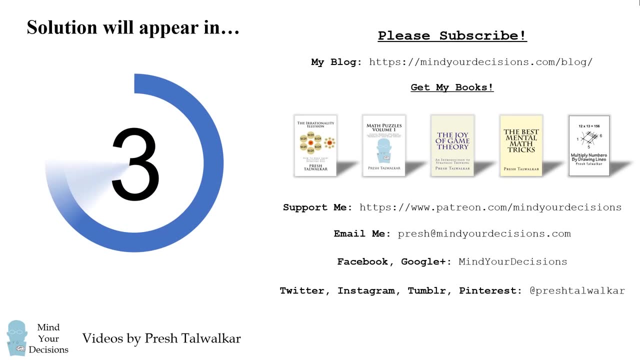 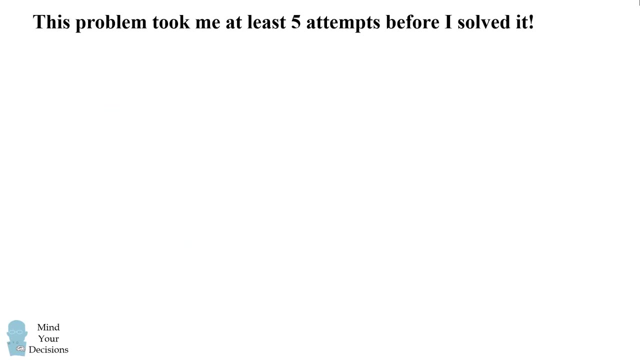 So I will say this problem was very challenging for me. But can you figure it out? Give this problem a try and when you're ready, keep watching the video for a solution. So this problem took me at least five attempts before I solved it. 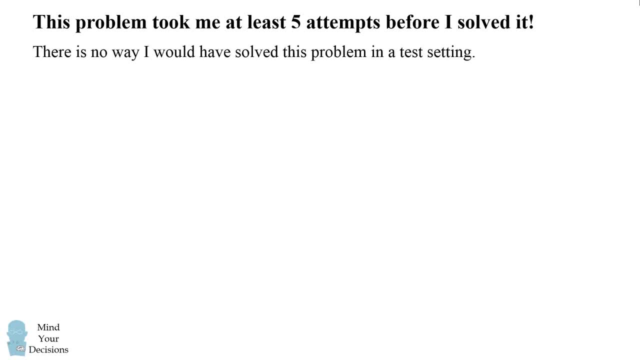 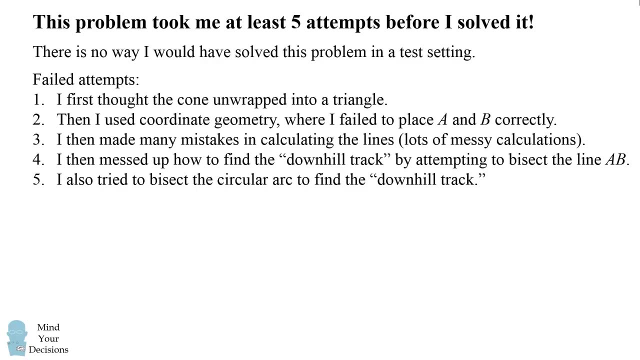 There is no way I would have solved this problem in a test setting, And here are some of the failed attempts. I first thought the cone unwrapped into a triangle. Next I used coordinate geometry, but I failed to put the points A and B in the correct positions. 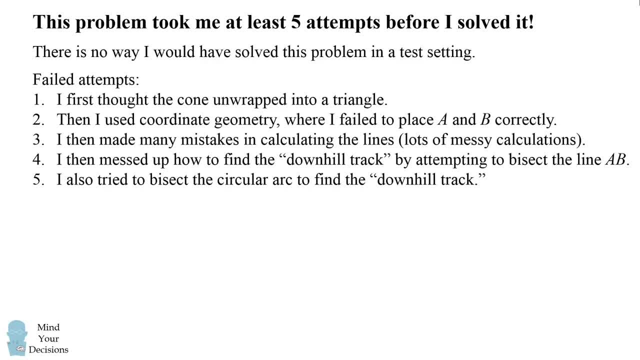 The third mistake is that I then made many mistakes in trying to calculate the equations of the lines. This led to many messy calculations. The fourth mistake is that I messed up how to find the length of the downhill track, because I tried to do it by bisecting the line AB. 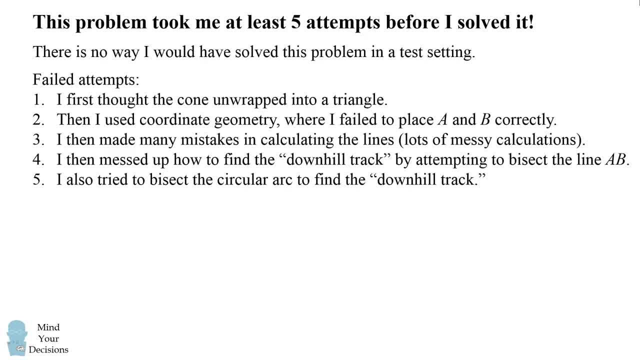 This is not correct. I then tried to solve it by bisecting the circular arc to find the downhill track. So I was stuck and then I said maybe I should try and find the answer on line. But then suddenly it hit me. Eventually I figured it out. 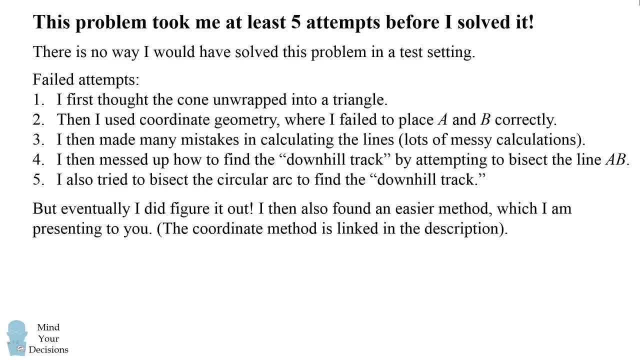 I then also found an easier method to solve the problem, which I am presenting to you. The coordinate method is linked in the description, So why am I sharing this story with you? The lesson is that don't give up if you can't solve a problem, And also don't peek at the video solution too early. 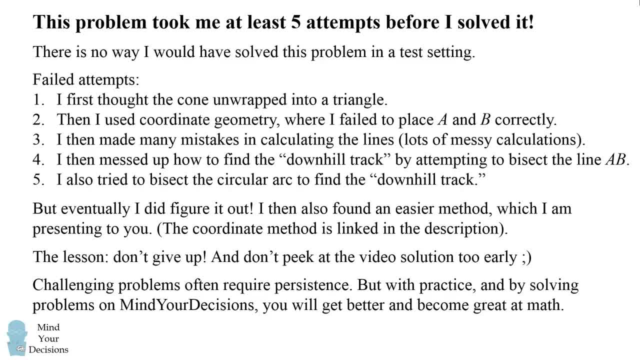 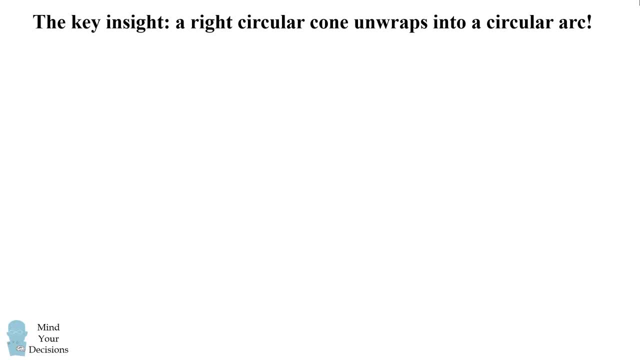 Challenging problems often require persistence, But with practice and by solving problems on mind your decisions- you will get better and you will become great. So how do we solve this problem? The key insight is that a right circular cone unwraps into a circular arc. 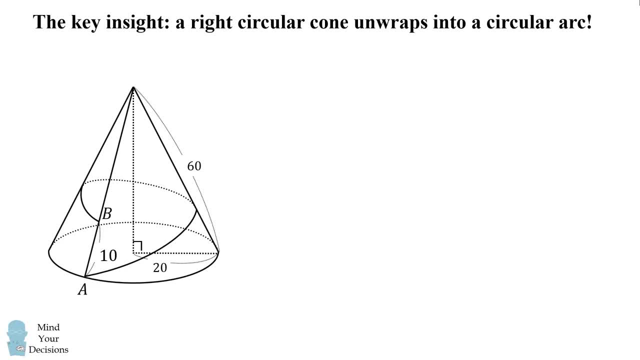 So here we have the cone-shaped mountain and let's just imagine a general cone. If you cut open a right circular cone, it will unwrap into a circular arc. So here's a visualization of what I'm talking about. So we have this cone. 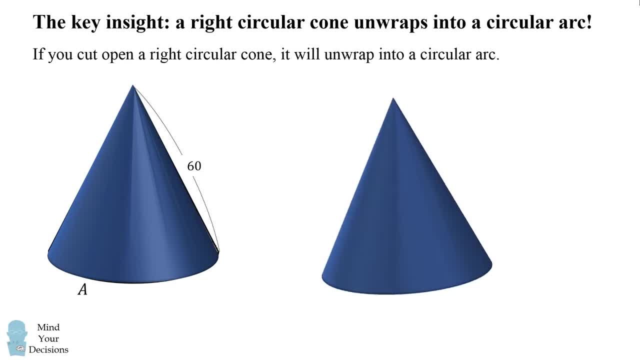 and it's a three-dimensional object. That makes the problem a little hard to visualize. It'll be a lot easier if we can make it two-dimensional. So let's imagine we're cutting this cone vertically in the front. What will happen if we unwrap the cone? 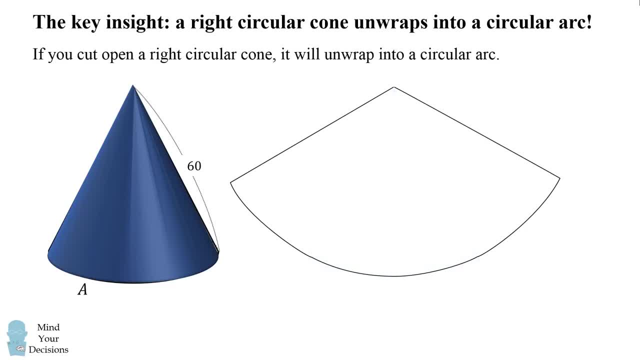 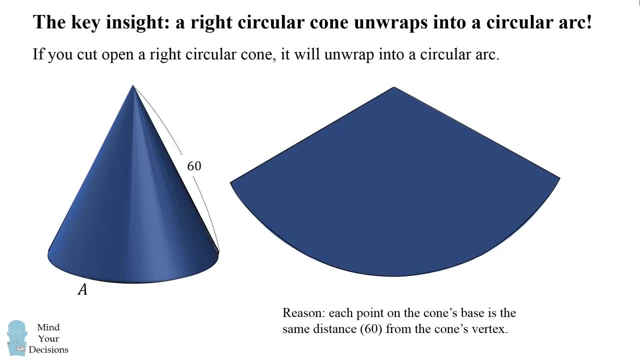 Wow. So this cone turns into a perfect circular arc. Now why is it a circular arc? The reason is that each point on the cone's base is the same distance of 60 from the cone's vertex. So here's the cone's base, and at the top is the cone's vertex. 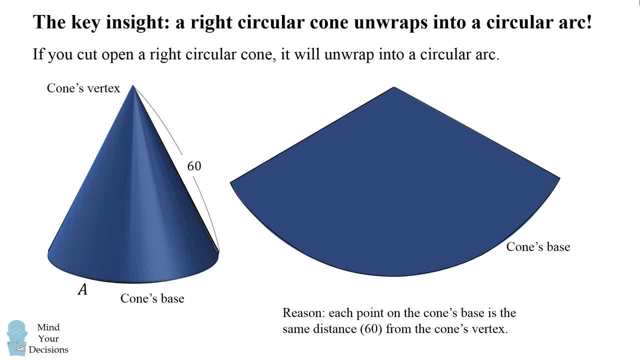 On the circular arc. we have the cone's base at the bottom and the cone's vertex at the top. Now each line on this cone's vertex to base this slant height exactly corresponds to a radius of this circular arc. So that's why we end up with a circular arc, because every distance from the 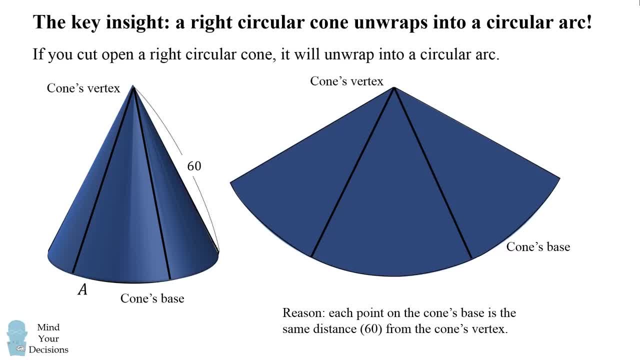 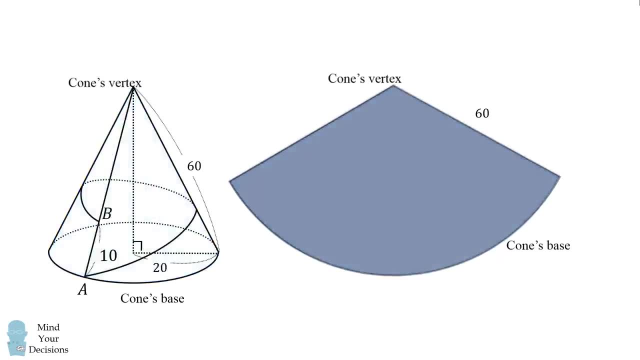 vertex to the base is the same slant height of 60. And so this circular arc has a radius of 60.. So now, how can we use this information to continue to solve the problem? Well, the first step is we're going to solve for the central angle of this circular arc. 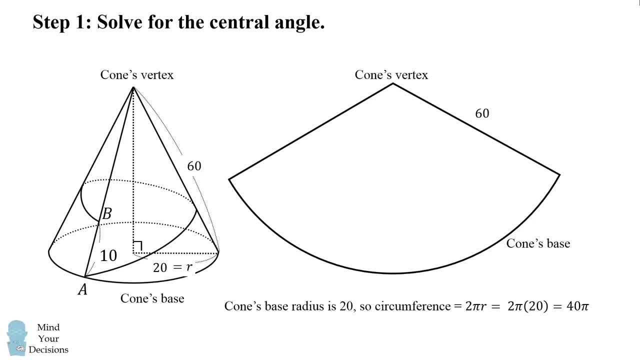 The radius of the cone's base is 60.. The radius of the cone's base is 20.. That means its circumference is 2 pi r, which is 2 pi times 20,, which is 40 pi. So that's the length of the circular arc. 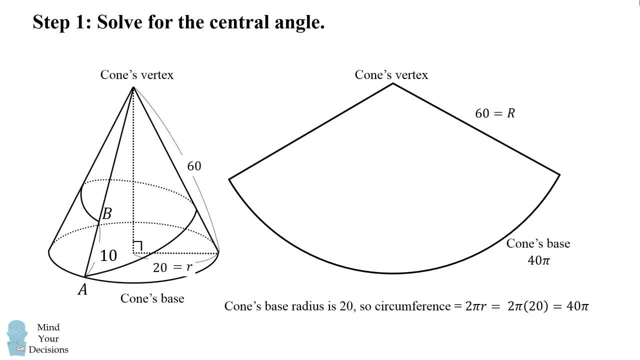 Now we know the radius of the circular arc is 60. This is capital R or the slant height of the cone. Now there's a formula that relates the radius of a circular arc, its central angle, to its length. So the length of the circular arc is R times theta. 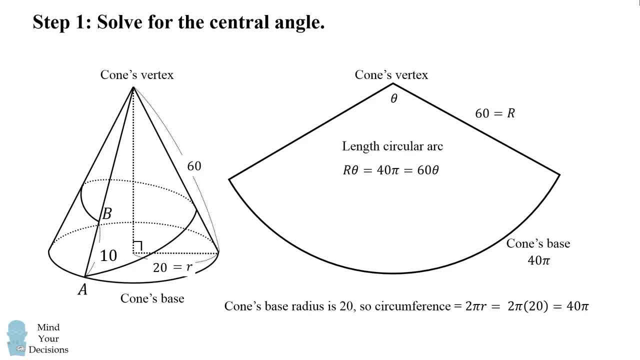 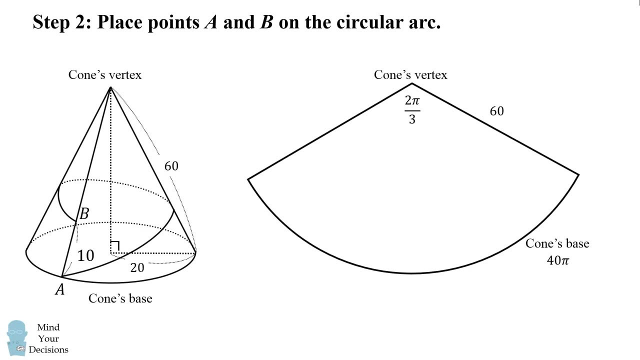 So here we know the length is 40 pi and R times theta is 60 theta. So we can solve that theta is equal to 2 pi over 3.. So that's the central angle. Next we will place points A and B on the circular arc. 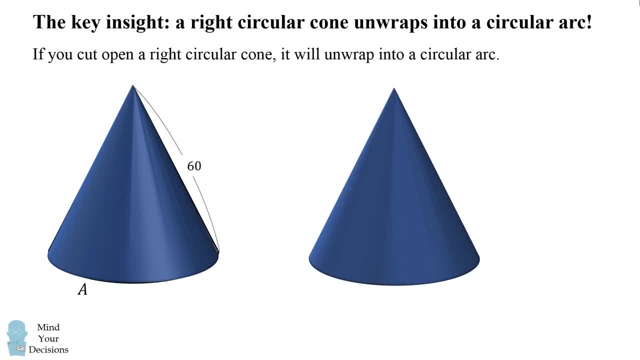 That makes the problem a little hard to visualize. It'll be a lot easier if we can make it two-dimensional. So let's imagine we're cutting this cone vertically in the front. What will happen if we unwrap the cone? Wow, So this cone turns into a perfect circular arc. 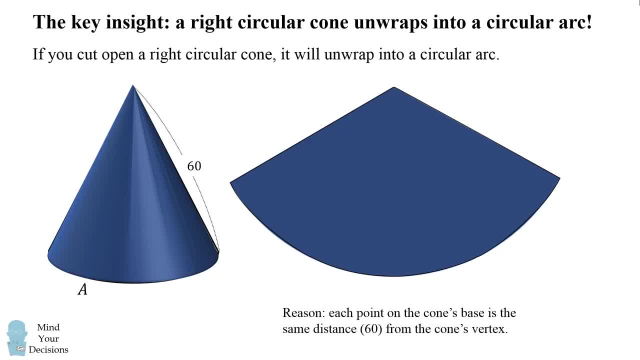 Now, why is it a circular arc? The reason is that each point on the cone's base is the same distance of 60 from the cone's vertex. So here's the cone's base, and at the top is the cone's vertex. 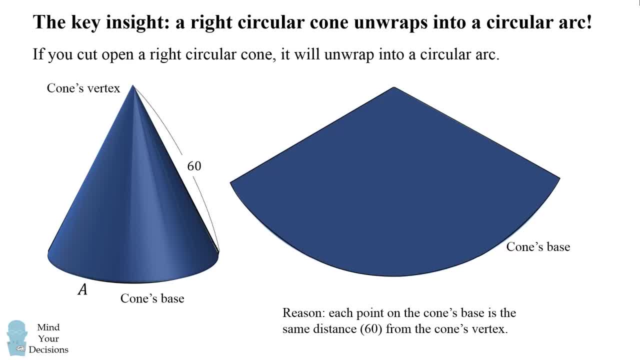 On the circular arc. we have the cone's base at the bottom and the cone's vertex at the top. Now each line on this cone's vertex to base this slant height exactly corresponds to a radius of this circular arc. So that's why we end up with a circular arc. 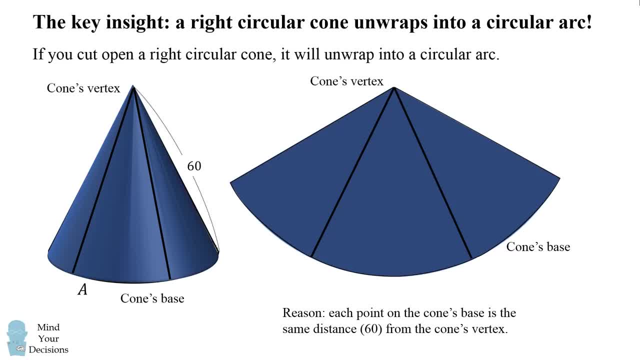 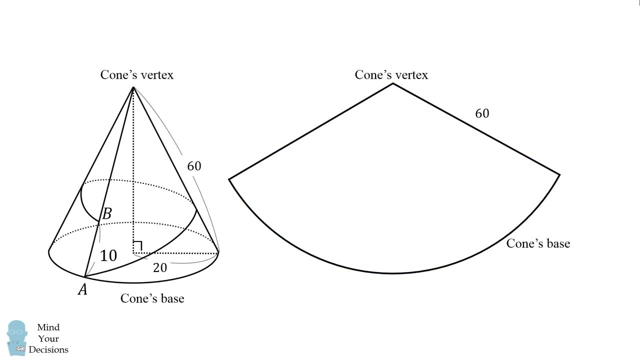 Because every distance from the vertex to the base is the same slant height of 60. And so this circular arc has a radius of 60. So now, how can we use this information to continue to solve the problem? Well, the first step is we're going to solve for the central angle of this circular arc. 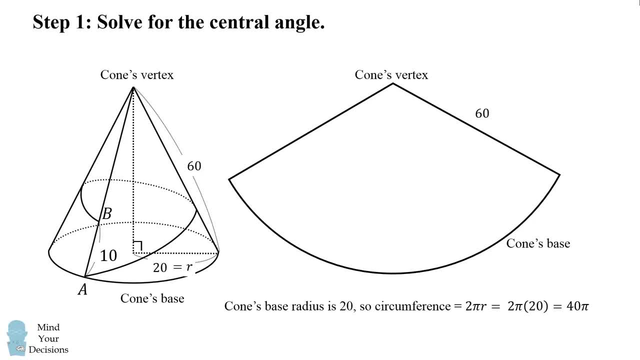 The radius of the cone's base is 60.. The radius of the cone's base is 60.. The radius of the cone's base is 60.. The radius of the cone's base is 20.. That means its circumference is 2 pi r, which is 2 pi times 20, which is 40 pi. 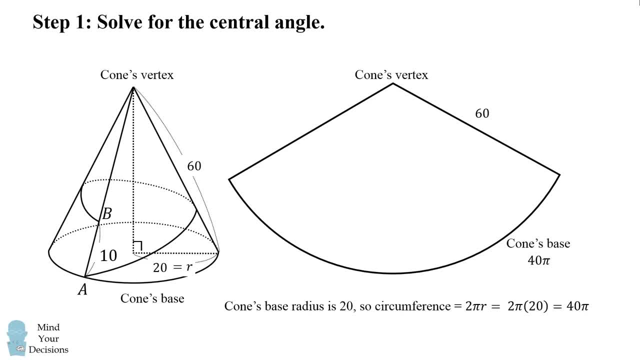 So that's the length of the circular arc. Now we know the radius of the circular arc is 60. This is capital R, or the slant height of the cone. Now there's a formula that relates the radius of the circular arc. 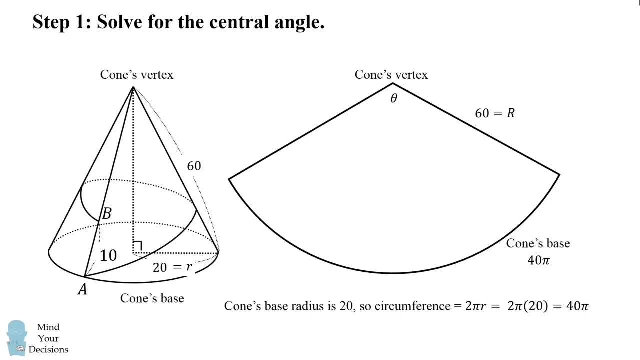 its central angle to its length. So the length of the circular arc is R times theta. So here we know the length is 40 pi and R times theta is 60 theta. So we can solve that theta is equal to 2 pi over 3.. 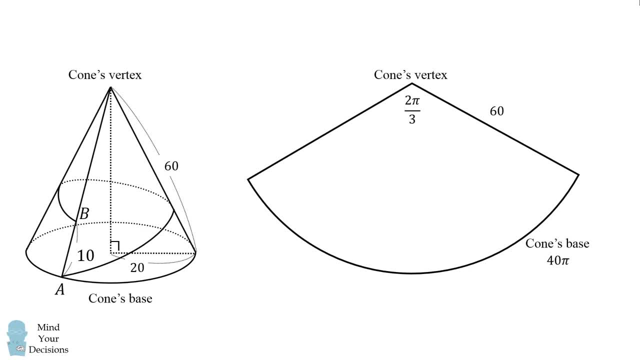 So that's the central angle. Next, we will place points A and B on the circular arc. So what happens then? So what happens when we unwrap this cone into a circular arc? Well, point A is along the base, So we know it'll have to be somewhere along the base of this circular arc, at the very edge. 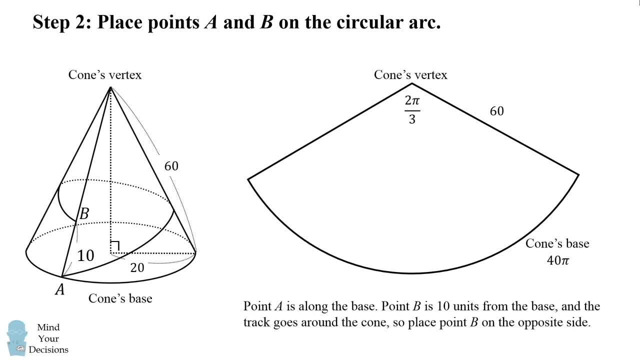 Point B is 10 units from the base and the track goes around the cone, So point B is going to be on the opposite side of where we place point A. So let's place point A on the right-hand side of the circular arc. 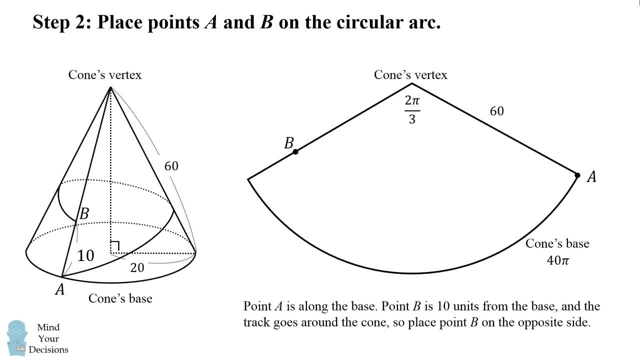 We want to place point B on the other side of the circular arc. We want to place point B on the other side of the circular arc. We want to place point B on the other side of the circular arc and 10 units away from the base. 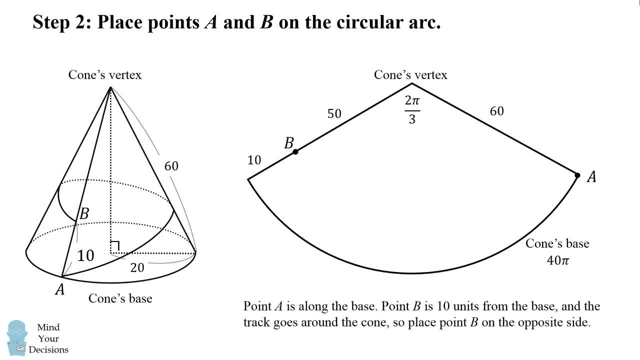 So it'll be 10 units from the end of the arc and it'll be 50 units from the vertex, because the radius is 60. Now, what's the shortest path from A to B? Well, in this circular arc, the answer is simple. 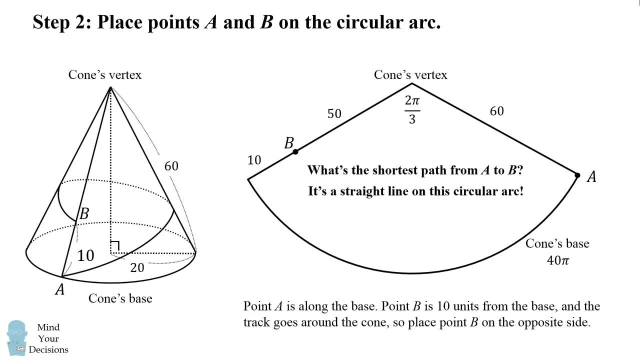 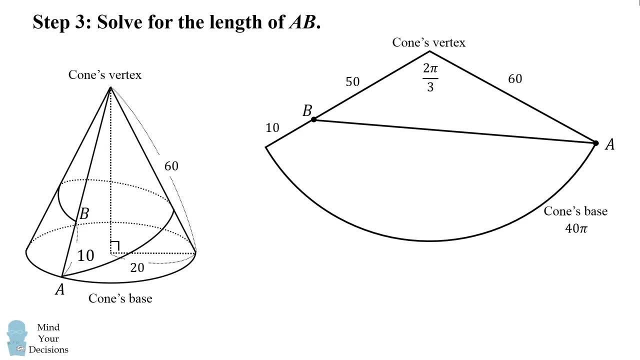 It's a straight line between points A and B. So now we're going to to solve for the length of AB. We draw a straight line between A and B. So how can we solve for this length? We can use a little bit of trigonometry. 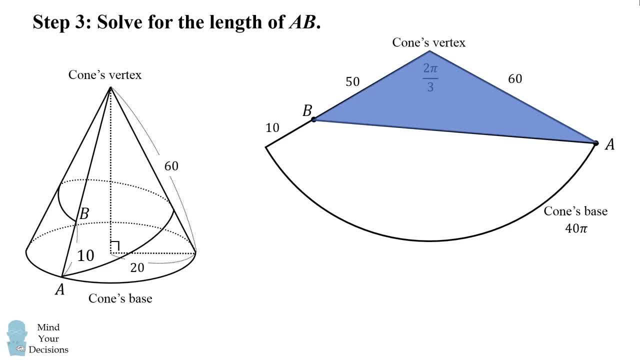 Let's consider this triangle. We know two of its lengths and we know the angle between those sides, So we can use the law of cosines to figure out the length of the third side. C squared is equal to A squared plus B squared minus 2AB times cosine of capital C. 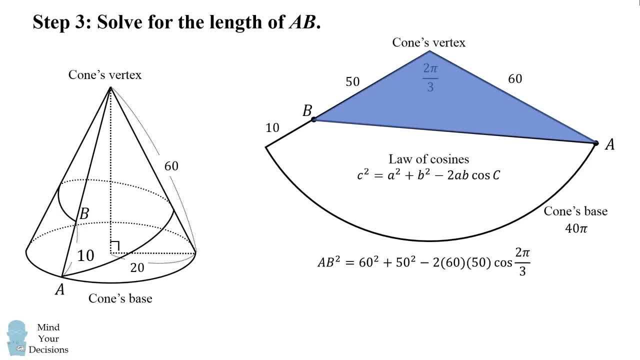 the angle between those two sides. So here we have. the length of AB squared is equal to 60 squared plus 50 squared minus 2 times 60 times 50 times the cosine of the central angle, 2 pi over 3.. We can simplify this to get: AB squared is equal to 9100,. 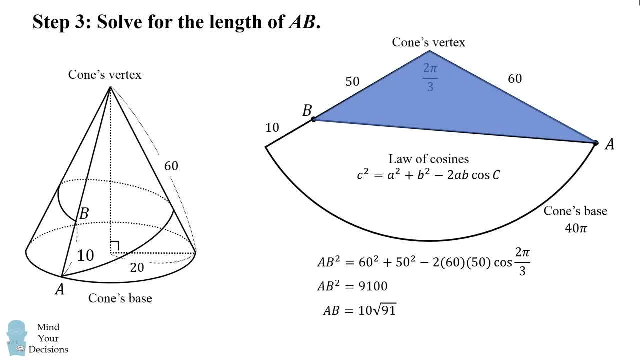 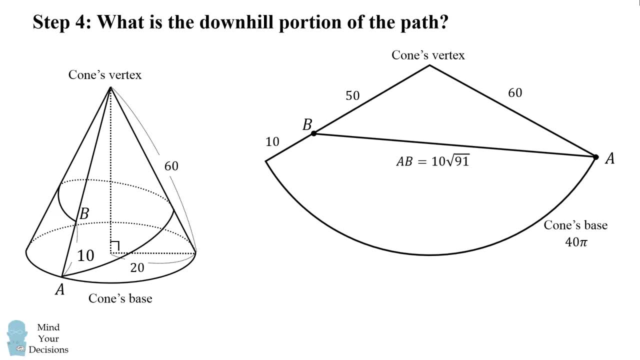 which means AB is equal to 10 times the square root of 91.. So we're making good progress, But now what is the downhill portion of AB squared? We know the total length of the track, but we're asked to figure out the downhill portion. 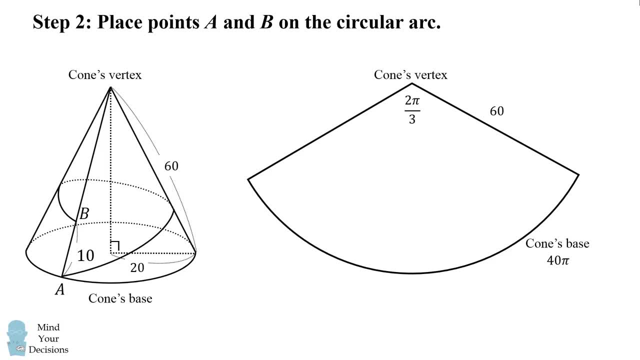 So what happens when we unwrap this cone into a circular arc? Well, point A is along the base, So we know it'll have to be somewhere along the base of this circular arc. at the very edge. Point B is 10 units from the base and the track goes around the cone. 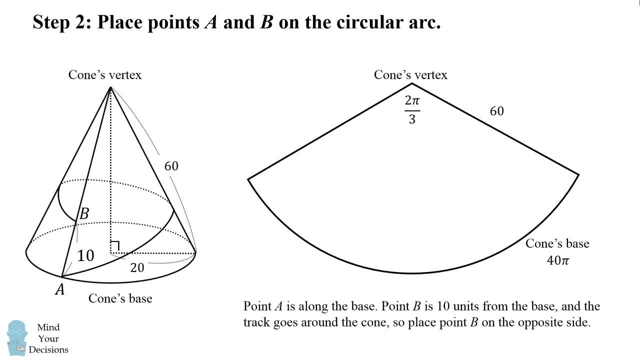 So point B is going to be on the opposite side of where we place point A. So let's place point A on the right-hand side of the circular arc. We want to place point B on the opposite side of where we place point A. 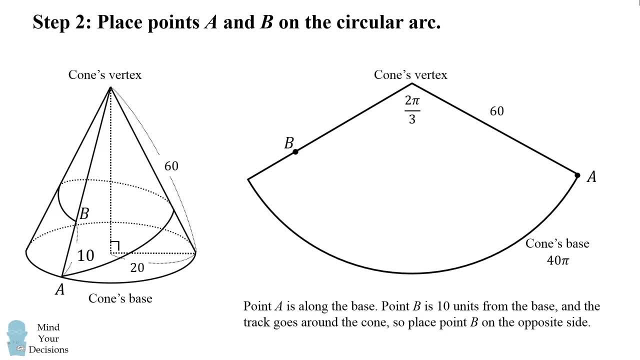 So it's going to be on the other side of the circular arc and 10 units away from the base. So it'll be 10 units from the end of the arc and it'll be 50 units from the vertex because the radius is 60.. 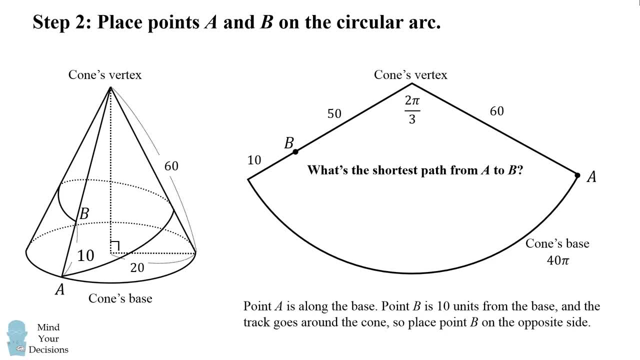 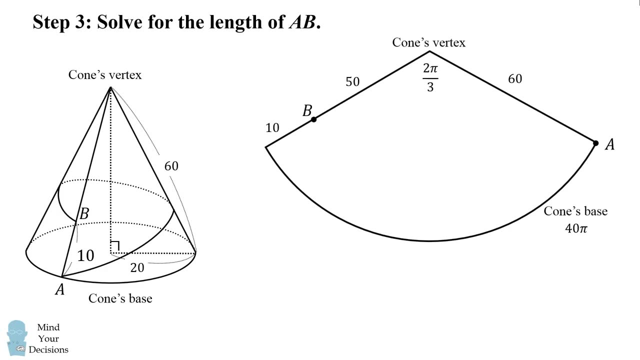 Now, what's the shortest path from A to B? Well, in this circular arc, the answer is simple: It's a straight line between points A and B. So now we're going to solve for the length of AB. We draw a straight line between A and B. 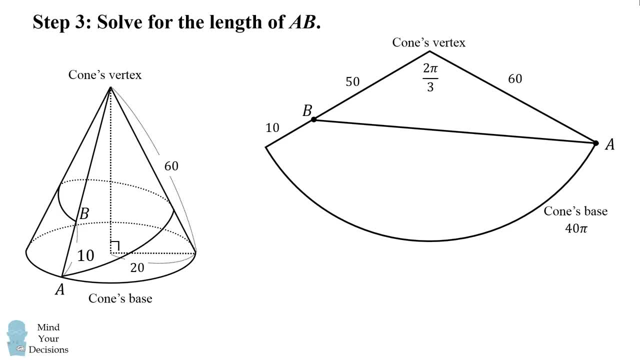 So how can we solve for this length? We can use a little bit of trigonometry. Let's consider this triangle. We know two of its lengths and we know the angle between those sides, So we can use the law of cosines to figure out the length of the third side. 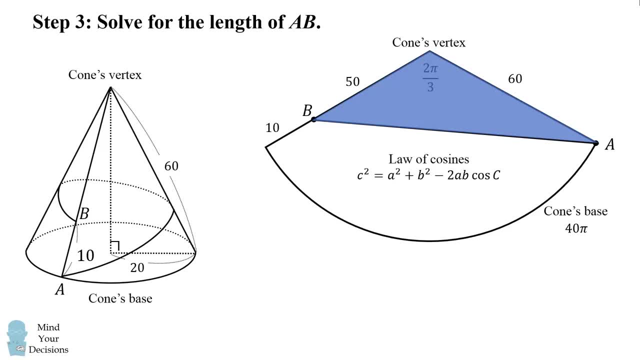 C squared is equal to A squared plus B squared, minus 2AB times cosine of capital C, the angle between those two sides. So here we have. the length of AB squared is equal to 60 squared plus 50 squared minus 2 times 60 times 50, times the cosine of the central angle: 2 pi over 3.. 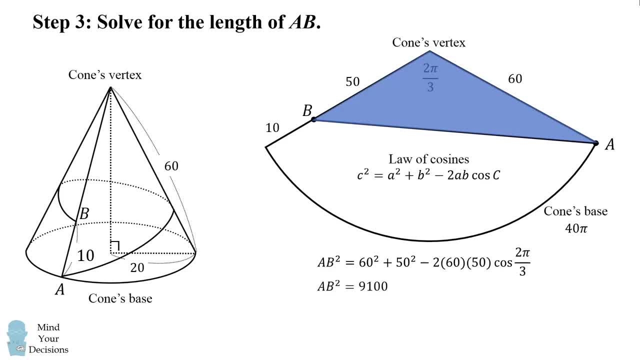 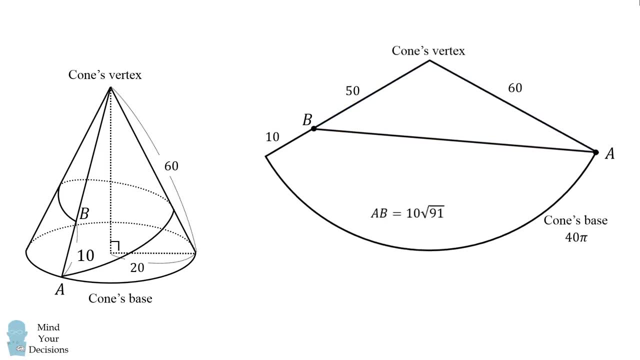 We can simplify this: to get AB squared is equal to 9100, which means AB is equal to 10 times the square root of 91. So we're making good progress. But now what is the downhill portion? We know the total length of the track, but we're asked to figure out the downhill portion. 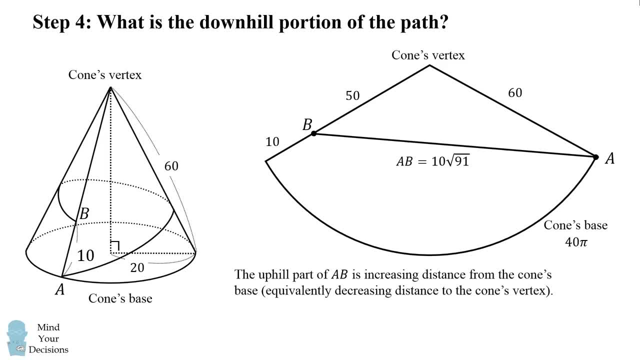 So the uphill part of AB is increasing distance from the cone's base, which is equivalently decreasing distance to the cone's vertex. The downhill part of AB is decreasing distance from the cone's base, which is equivalently increasing distance to the cone's vertex. 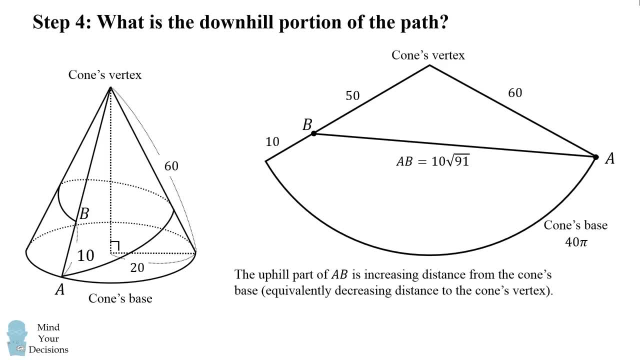 So the uphill part of AB is increasing distance from the cone's base, which is equivalently decreasing distance to the cone's vertex. The downhill part of AB is decreasing distance from the cone's base, which is equivalently increasing distance to the cone's vertex. 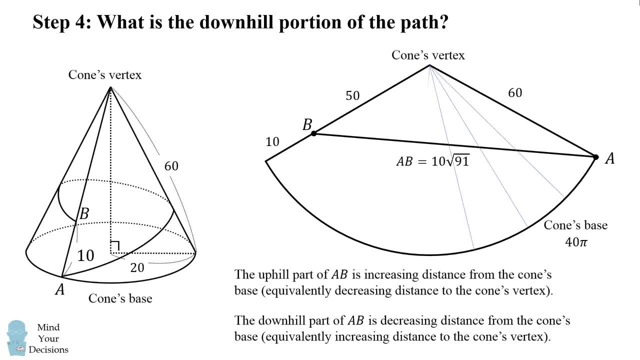 So if we draw some slant heights, which will be represented as radii, on this circular arc, the uphill portion will be decreasing distance to the cone's vertex and then the downhill part will be increasing. Furthermore, the downhill part of AB begins when the line is closest to the cone's vertex. 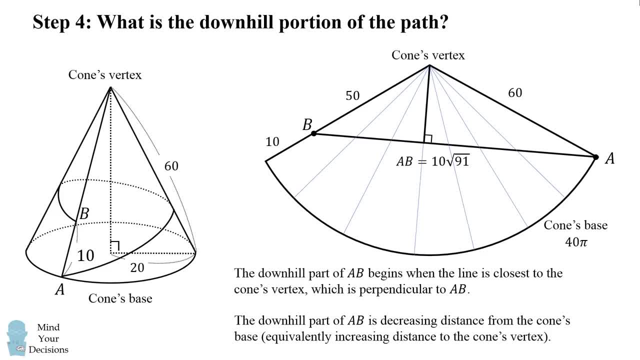 and that'll be perpendicular to AB. So this will be the point at which the track goes from going uphill to going downhill. Now we are already given that the track goes from uphill to downhill and I use that information to then say we'll look for the perpendicular. 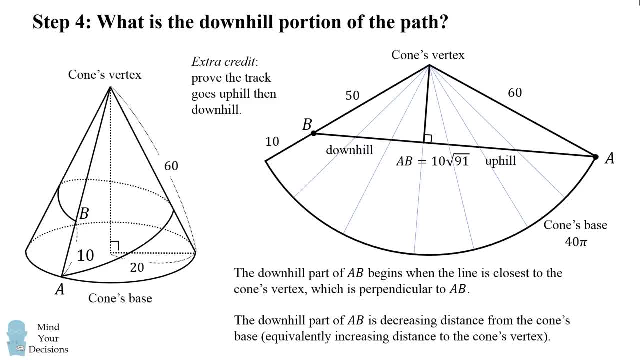 and this has to be the point. But to truly prove this problem for extra credit, you can prove that the track goes uphill and then downhill, And I'm sure some of you who think all these problems are true. you can prove that the track goes uphill and then downhill. 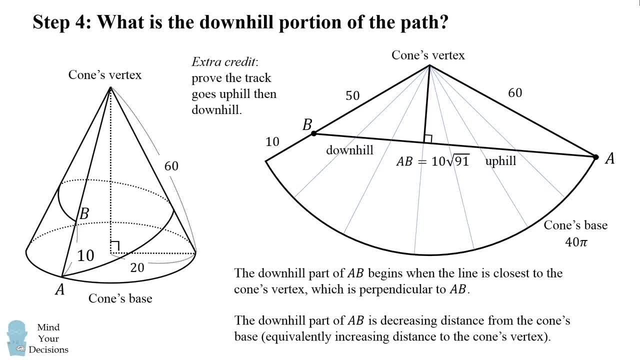 And I'm sure some of you who think all these problems are true- you can prove that the track goes uphill and then downhill. We'll be able to figure this out. You know it won't be very difficult for you, but it's actually a little bit of a complicated thing to show. 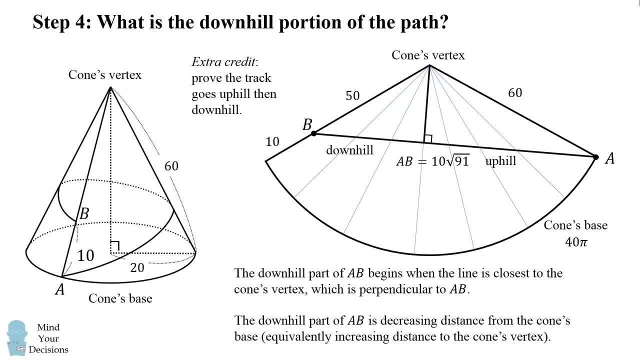 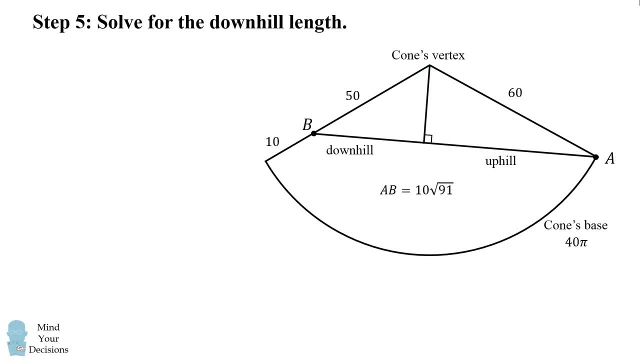 Anyway, this is a test question. We're going to use this information that was given to us and then continue to solve the problem. So now, how do we figure out the downhill length? We again use some geometry. Let's label the downhill portion x. 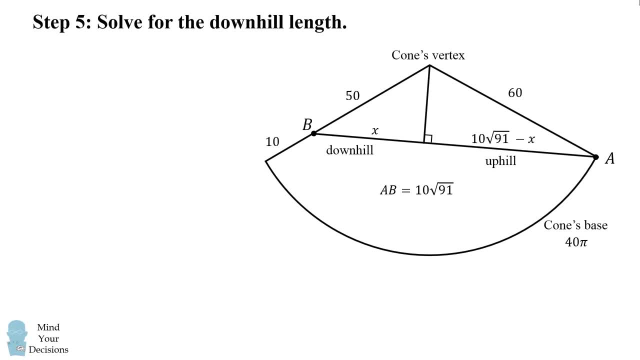 The uphill portion will be 10 squared to 91.9.. The uphill portion will be 10 squared to 91.9.. Minus x, And let's label the distance from the vertex to the line AB as h By the Pythagorean theorem. in one triangle, the uphill portion. 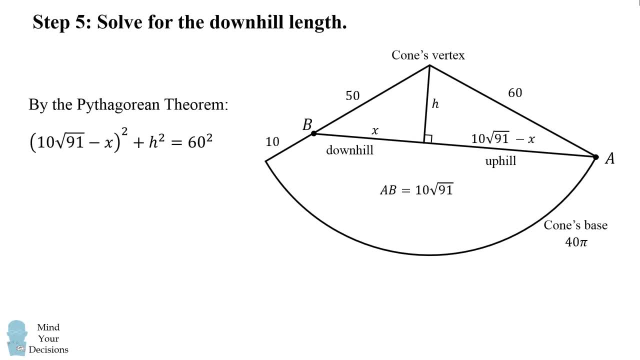 we have the quantity 10 times the square root of 91, minus x squared, plus h squared is equal to 60 squared. And in the downhill triangle we have x squared plus h squared is equal to 50 squared. Now there's a neat trick. 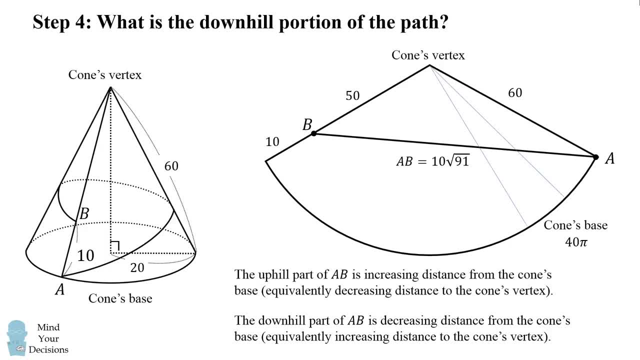 So if we draw some slant heights, which will be represented as radii, on this circular arc, the uphill portion will be decreasing distance to the cone's vertex and then the downhill part will be increasing. Furthermore, the downhill part of AB begins when the line is closest to the cone's vertex. 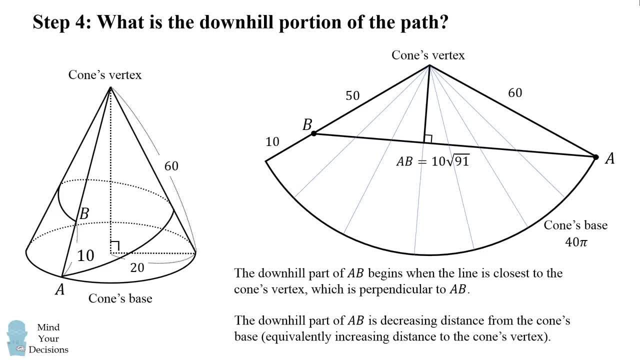 and then will be perpendicular to AB. So this will be the point at which the track goes from going uphill to going downhill. Now we are already given that the track goes from uphill to downhill and I use that information to then say: we'll look for the perpendicular. 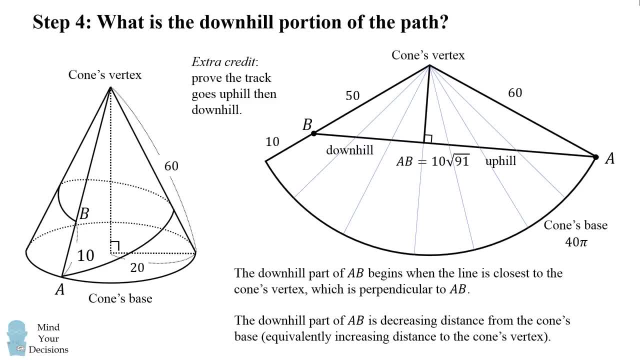 and this has to be the point. But to truly prove this problem for extra credit, you can prove that the track goes uphill and then downhill, And I'm sure some of you who think all these problems are easy, will be able to figure this out. 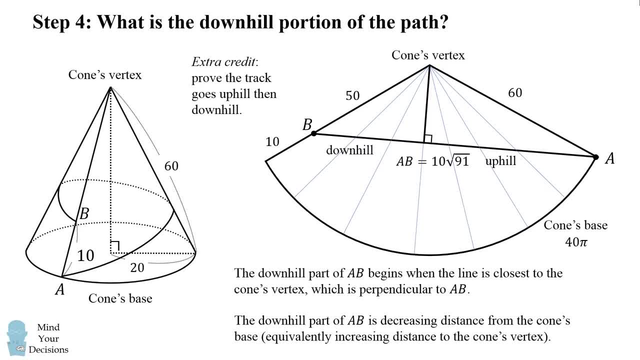 You know it won't be very difficult for you, but it's actually a little bit of a complicated thing to show. Anyway, this is a test question. We're going to use this information that was given to us and then continue to solve the problem. 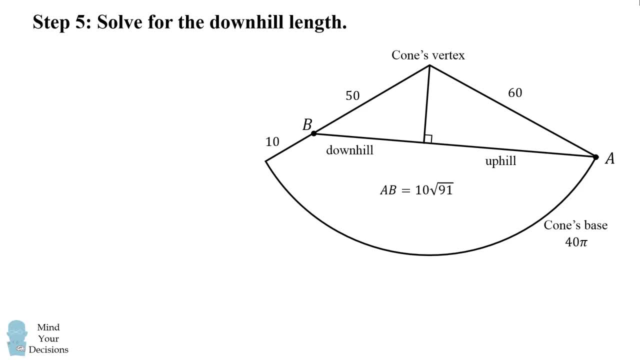 So now, how do we figure out the downhill length? We again use some geometry. Let's label the downhill portion x. the uphill portion will be 10 squared to 91 minus x. and let's label the distance from the vertex to the line AB as h. 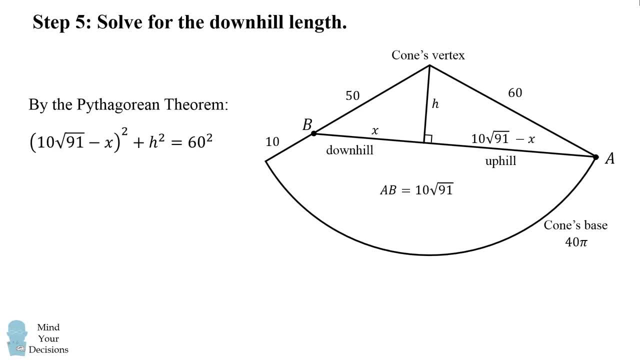 By the Pythagorean theorem. in one triangle, the uphill portion, we have the quantity 10 times the square root of 91 minus x squared plus h squared is equal to 60 squared. and in the downhill triangle we have x squared plus h squared is equal to 50 squared. 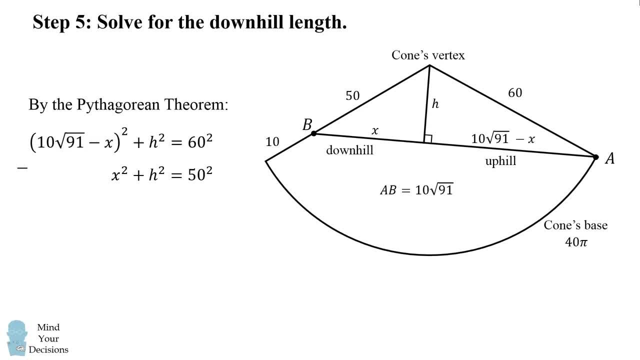 Now there's a neat trick: We can subtract this second equation from the first and we'll cancel out the h squares and we'll also cancel out the x squares. So this will simplify to be 9100 minus 2 times, 10 times the square root of 91 times x.